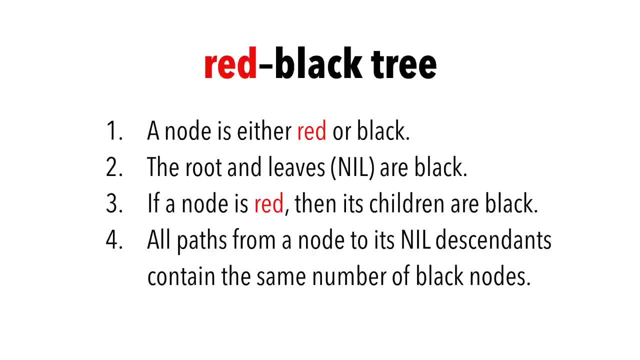 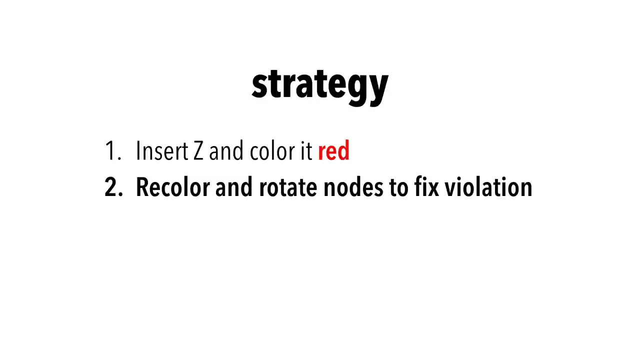 properties. By coloring the node red we may break property 2 or 3, but it turns out these violations are fairly easy to fix and you will see how Let's break down step 2 in our strategy After we insert the node and color it red. 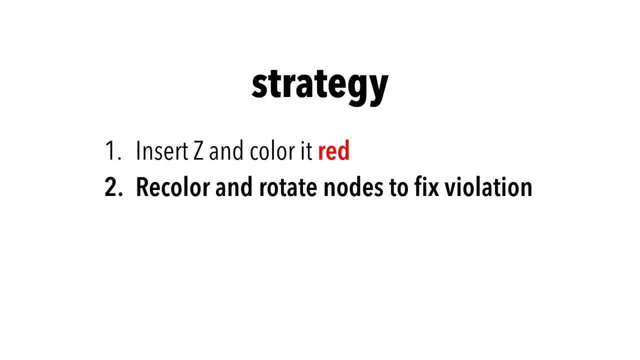 there will be four main scenarios we can encounter that will need further attention. Z could be the root, Z's uncle might be red and Z's uncle might be black. There are two different cases when Z is a black element. If the node and its generation table address are the same, then you. 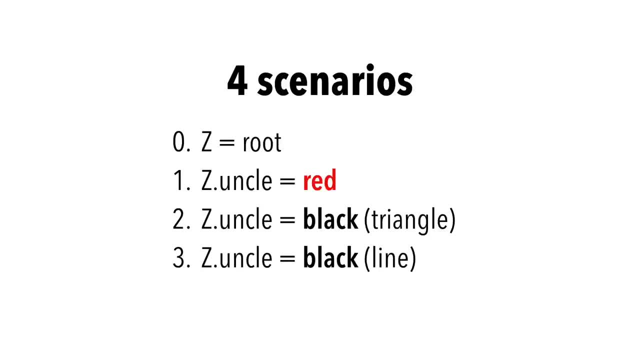 might need to lock down the node, which would be pink, or if the node and its generation table address uncle. For now, ignore the triangle and line part in parentheses. We'll cover those later. Let's discuss Case 0, when Z is the root. This one is pretty simple. All we need to do is color Z. 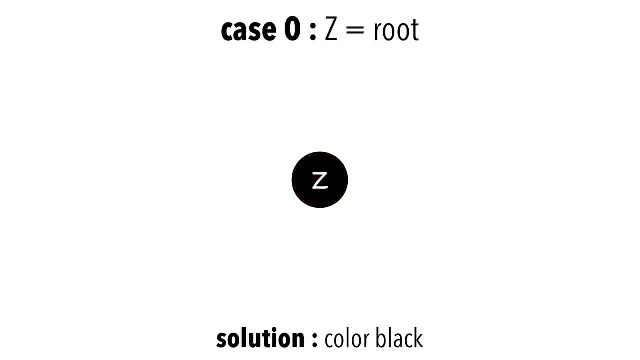 black. Moving on to Case 1, when Z has a red uncle. For this situation, we recolor Z's parent, grandparent and uncle. You might be wondering why B is red- the root of the tree. Just note that this is a subtree. You'll see Case 1 as part of a larger tree in the example video. 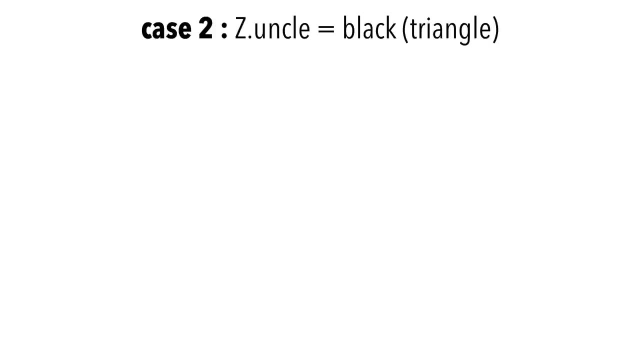 Case 2 is when Z's uncle is black, with triangle as the identifier. Let's say: this is our graph C is black and is Z's uncle. This is what I mean by triangle Z, Z's parent and Z's grandparent form a triangle. This is because Z is a left child. 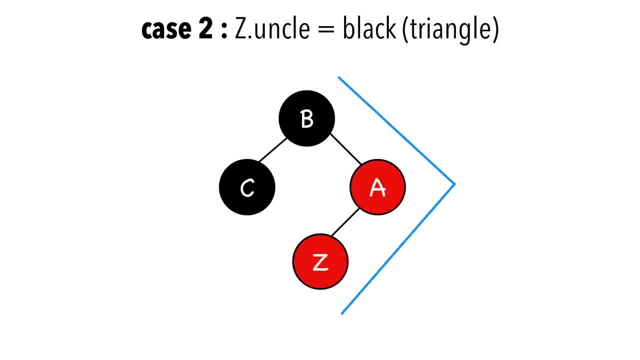 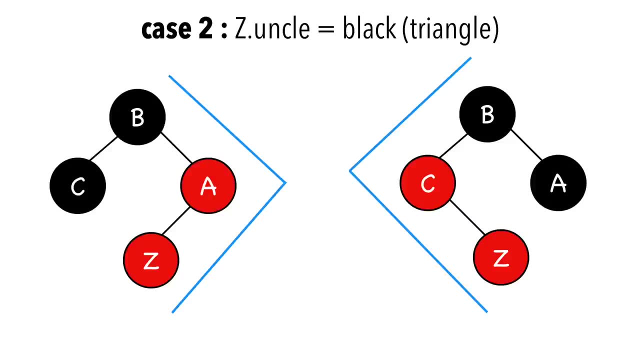 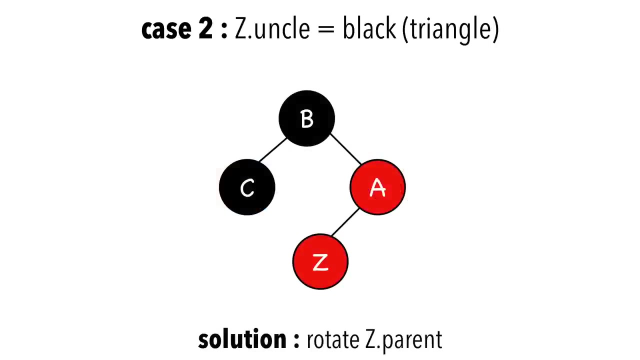 and its parent, A, is a right child. You might also see the triangle case like this, where Z is a right child and its parent is a left child. Same thing, just symmetrical. When we encounter this case, we rotate Z's parent, doing so in the opposite direction of Z, so Z takes. 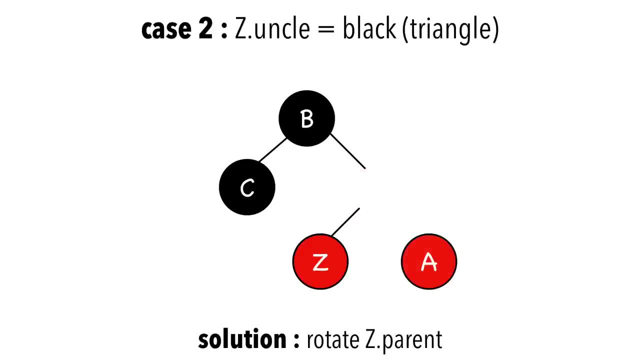 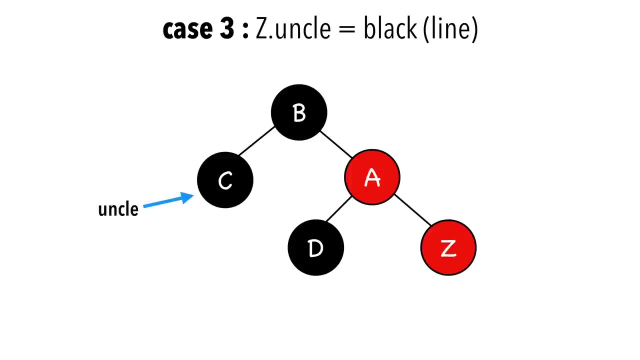 the place of A Nothing too tricky. Finally, Case 3 is when Z's uncle is black, with line as the identifier. Again, C is Z's uncle, but, as you can see, Z, Z's parent and Z's grandparent form a line. That's because Z is. 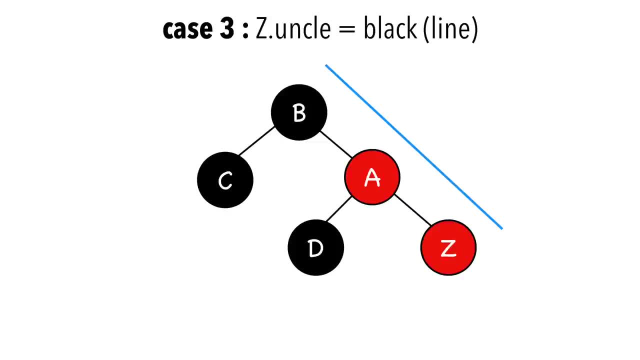 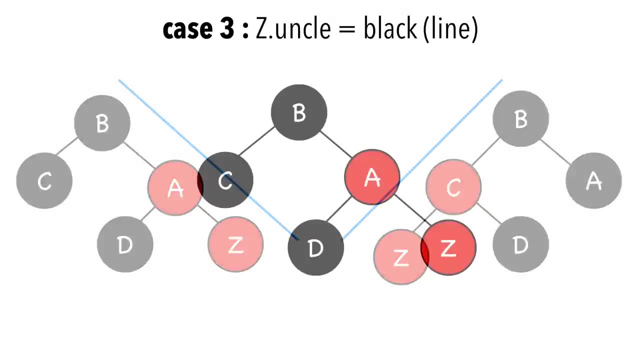 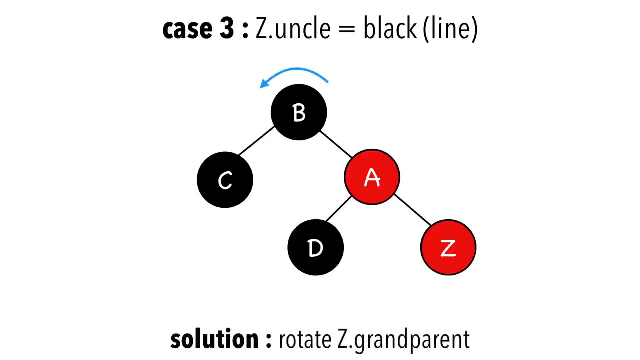 a right child and so is its parent, A. The symmetrical situation is when they are both left children. For Case 3, we rotate Z's grandparent again in the opposite direction of Z, so that A takes the place of B. 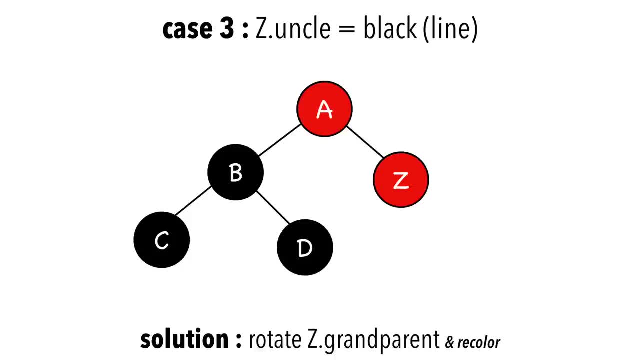 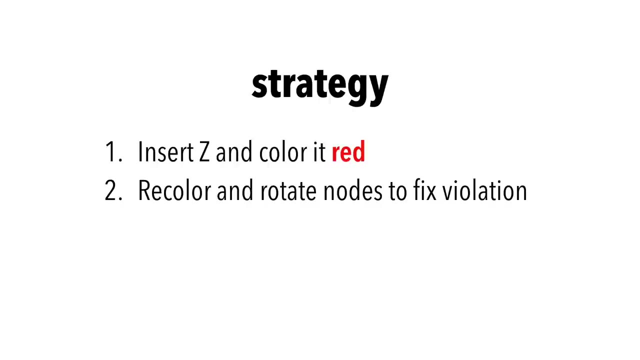 For Case 3, you will need to recolor the original parent and grandparent after the rotation. That's it. Let's review quickly. To start, we insert the node and color it red. Red-black trees have certain standards, so we must recolor and rotate nodes to fix violations. 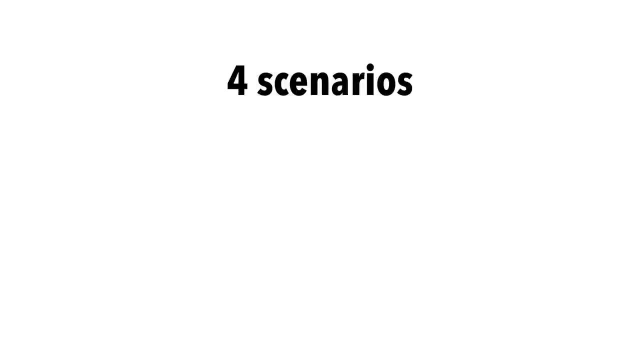 There are four possible fixes we'll encounter. First, when Z is the root, we color it black. Second, when Z's uncle is red, we recolor it black. Third, we recolor Z's parent, grandparent and uncle. 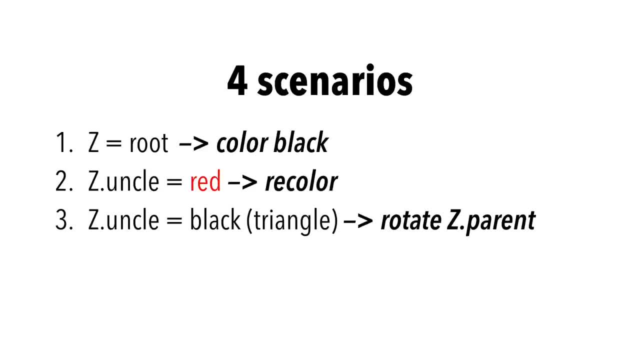 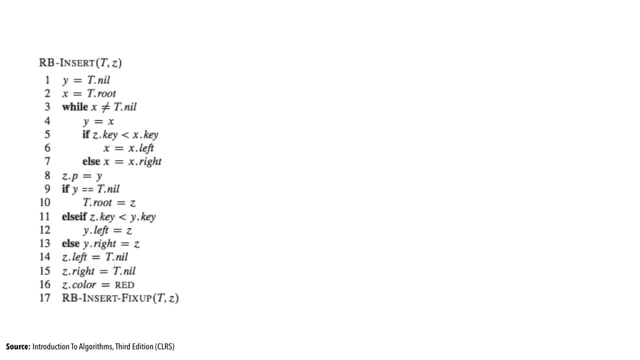 When Z's uncle is black and a triangle is formed, we rotate Z's parent, And when Z's uncle is black and a line is formed, we rotate Z's grandparent and do some recoloring. Here's the pseudocode for your reference. 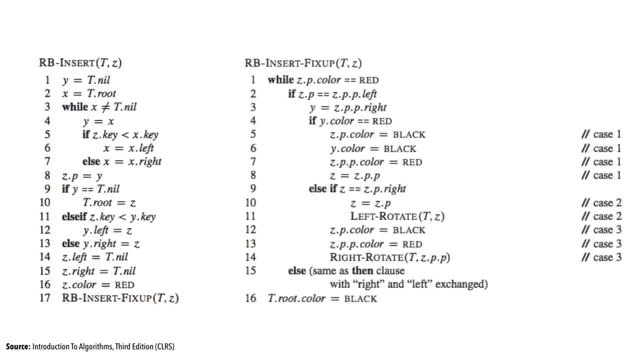 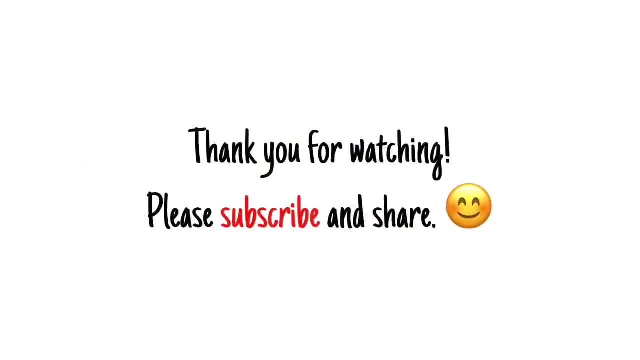 RBInsert is simply inserting the node. RBInsertFixup covers our four scenarios. Stay tuned for next time. You'll see our strategy in action as we walk through some examples. Thank you for watching. Please subscribe if you learned something.